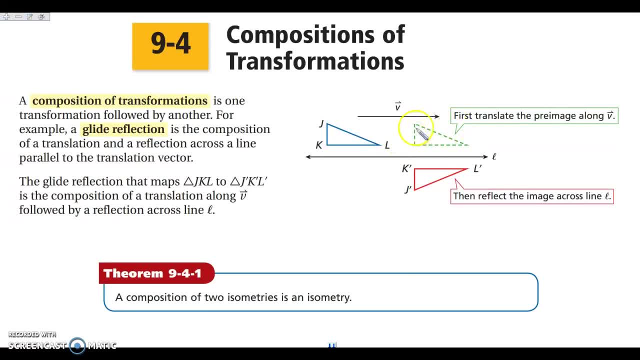 label this one as j prime, k prime, l prime. then you could use double primes, which would look like this in order to help you determine, because sometimes it's easier, as you're doing multiple transformations, to keep track of your transformations along the way by giving them. 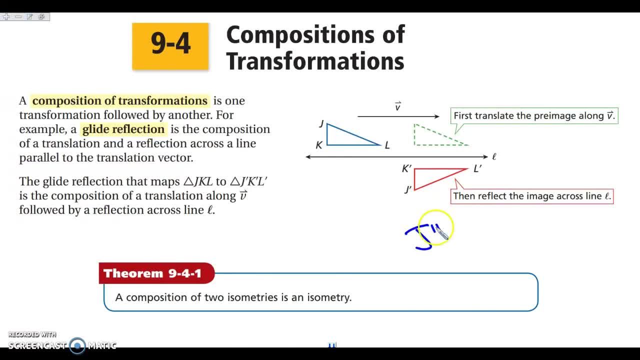 the same letters. So what you can do is just add multiple primes for multiple transformations. Okay, anytime we have more than one isometry, our final transformation is still an isometry, meaning if you never change the size or shape of the figure, then your final figure is going to be the same size and shape as your initial figure. 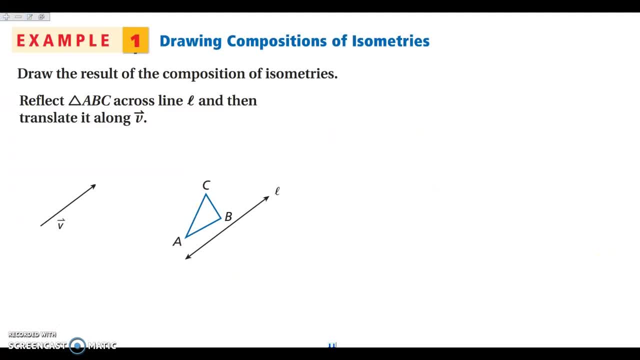 So when we take a look at example one, so with example one, we're going to draw our glide reflection to the same size and shape as your initial figure. We're going to create a slide for it. So here we have an idol, just. 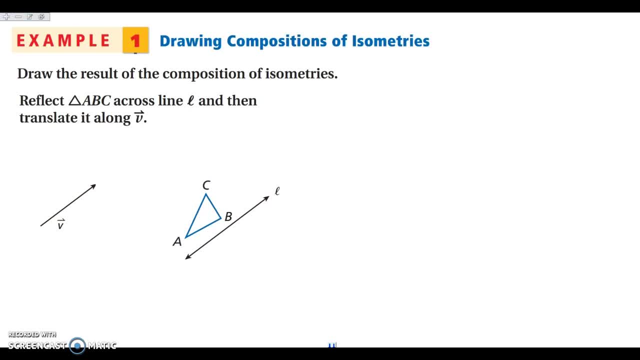 to help us understand that it's true. For example, here we have an arch and a miter here and we're also going to be using like a medium line here which will defy the boundary for the Shooting new player. but I'm going to похож upon this one for one. of these two options. One of these options is represented byرفlections. The other one is called line l, The other one is called line d. Okay, When we take our reflection here, we want to. well, actually we're going to do a reflex and then a glide. 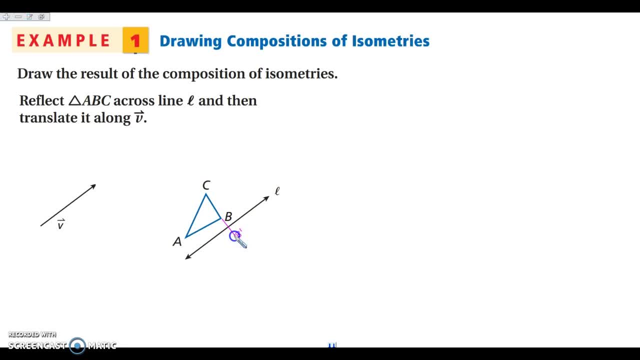 as B prime here. actually, let me move that a little bit, okay. so this point here is going to be B prime. then I'm going to repeat here: I want, I'm going, okay. so it's about this distance to the line. I want to try and match that on the. 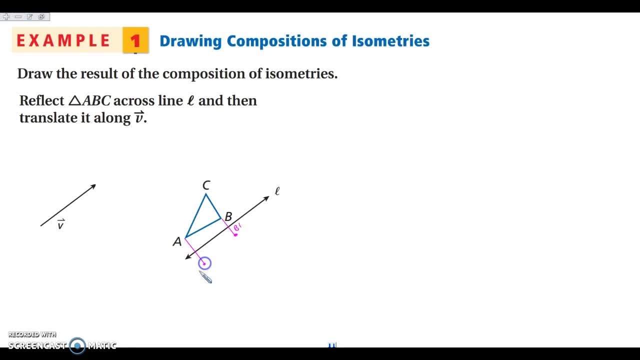 other side so that I can get my a prime. and then again we're gonna repeat that from C to the line and we want to go about the same distance again from the other side. so right about here is my C prime, because this is not my final image. 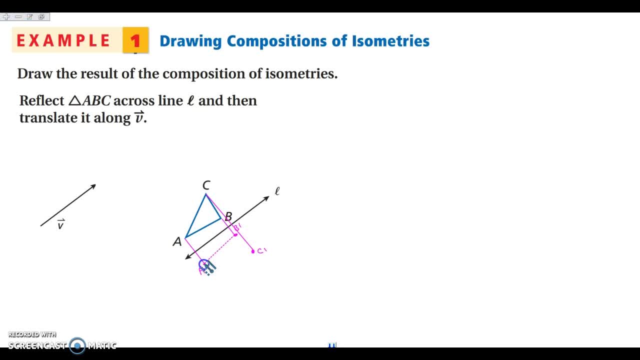 I am going to go ahead and dot it, so that way I know that this is not done yet. then the next thing that I want to do is I want to refocus, refocus, reflect it or, excuse me, translate it along this vector right here for V. so I 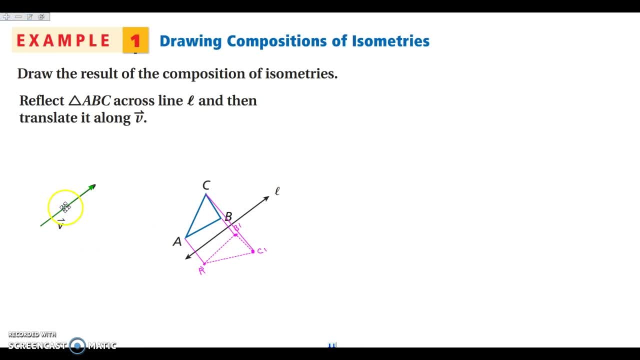 am going to take my vector and again, you guys can use that piece of paper trick that I showed you in class where you trace the vector with your piece of scratch paper, then flip that over and draw pencil on the back and then flip your paper back over and try and line it up. 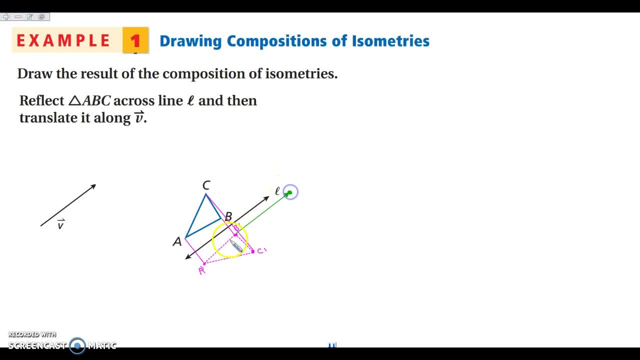 so I can have the ability here to just slide this vector around, but you should be doing that piece of paper trick that I showed you in class. okay, so this is gonna be from here. I'm moving my be here, so this is B double prime. this is what I. 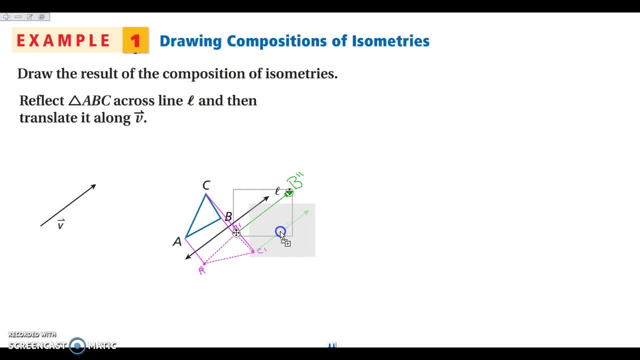 was kind of just talking about. then I'm gonna take my vector and I'm going to slide it over here to see so now that this is gonna be C double prime, and then I'm gonna take my vector here And I'm going to put it on A prime so that I can translate this here to get a double prime. 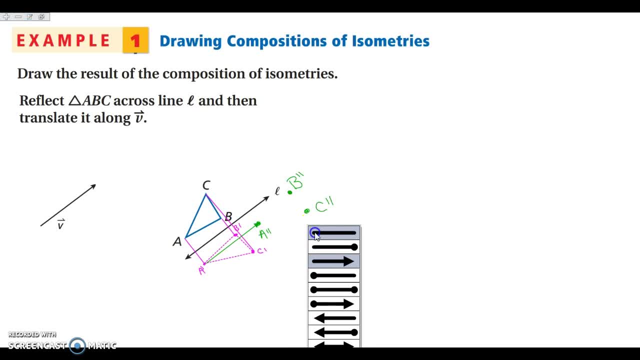 This is my final shape, And sometimes it's also nice to just kind of color it in. So a lot of times you'll see me, especially when we're doing like worksheets and stuff like that. Sometimes it gets a little hard when you're graphing to do this. 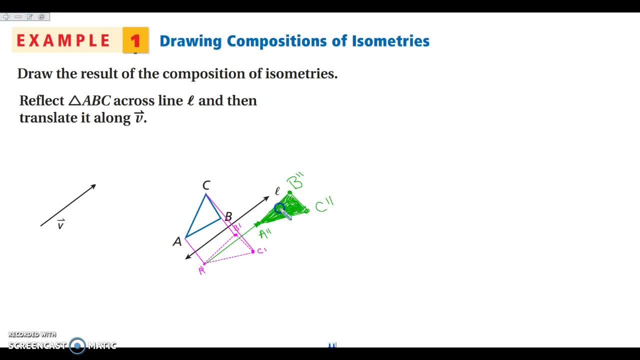 So I'm going to shade this one in so we know that this is the final one. So when you're doing yours, just make sure I can tell which one is your final one, Either by you coloring it in or by having all of your other ones just kind of dotted. so I know that you're not done yet. 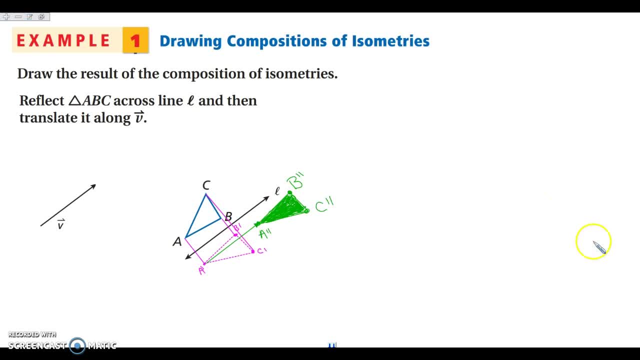 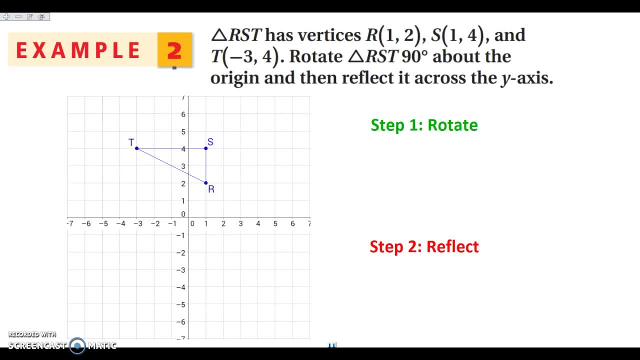 Okay, if you have any questions on that, go ahead and copy it on to your note taking guides now. Okay, so now we're going to take a look at what happens When we have- we're doing our multiple transformations here on a coordinate plane. 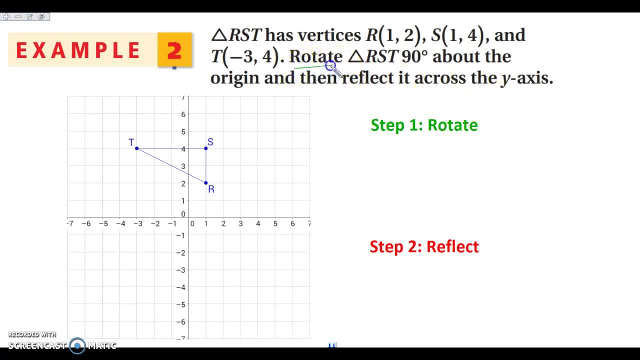 Sorry, Okay. so the first thing that I'm going to do is I want to rotate it 90 degrees and then we're going to reflect across the Y. So when I think back about my rotations, the first thing that I want to remember is what was my rotation rule. 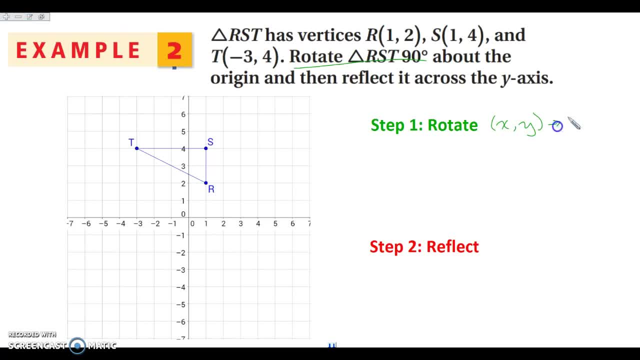 So my rotation rule was X. Y is going to map onto, So for rotating 90 degrees, that mapped onto negative Y comma X. So the first thing that I'm going to do is I'm going to write my original ordered pairs. R is at 1, 2.. 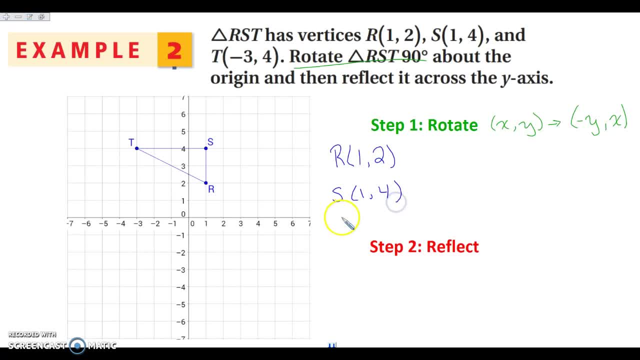 S is at 1, 4.. And T is at negative 3, 4.. So then when I am rotating it- R prime, S prime and T prime- I switch my values and I'm negating that Y, So this becomes negative 2, 1.. 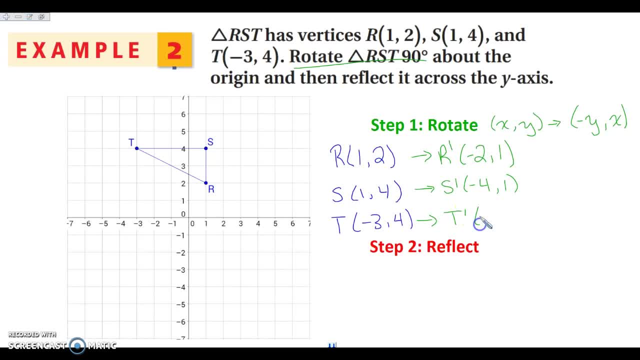 Negative 4, 1. And negative 4, negative 3.. So I'm going to go ahead and plot that now. So negative 2, positive 1.. So this is R prime And then S prime is negative 4, 1.. 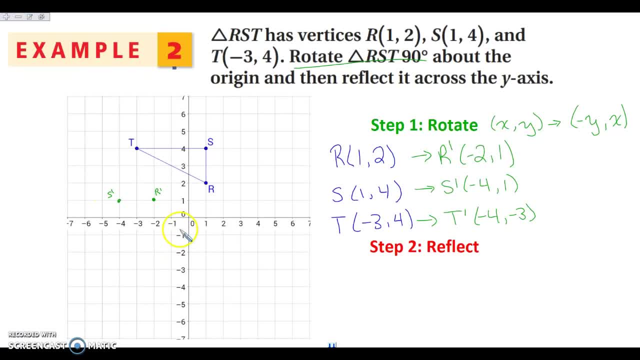 So this is going to be S prime, And then T prime is negative 4,, negative 3, which is right here- T prime. So, again, because this is not my final transformation, I'm just going to go ahead and dot this triangle. 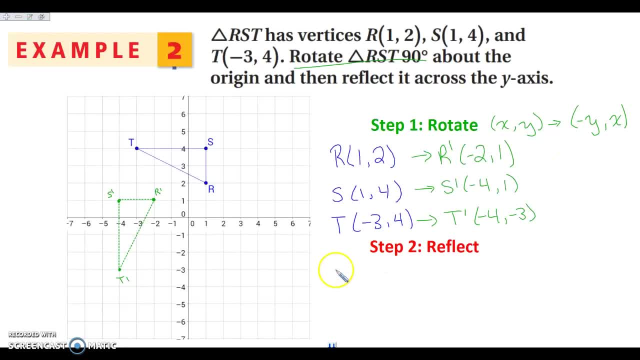 Then I'm going to kind of rewrite my points down here. R prime was at negative 2, 1.. S prime is at At negative 4, 1.. And T prime is at negative 4, negative 3.. Okay, then the next step is to reflect. 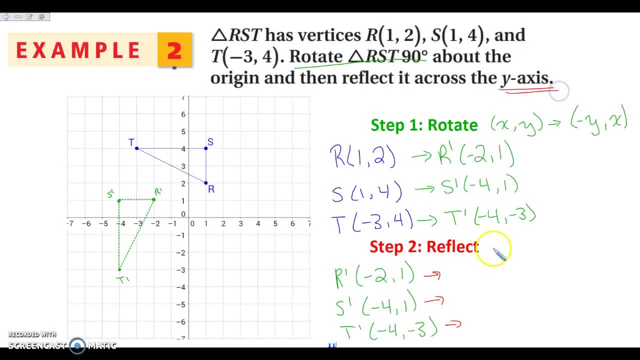 I am reflecting it across the Y axis, So my reflection rule for the Y is that XY is going to map onto negative X, Y. So all I'm doing here- Excuse me- Is negating my X values. So negative 2 becomes positive 2.. 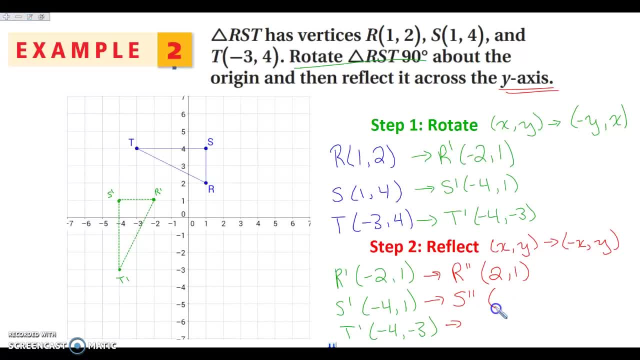 So this is 2, 1 for R double prime, S double prime is going to be 4, 1.. And T double prime is going to be 4, negative 3.. All right, So then we're going to go ahead and graph that. 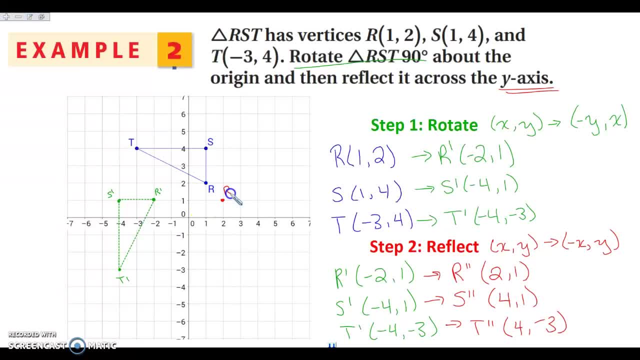 So we have 2, 1 here for R double prime, And then we have 4, 1.. 4, 1 is going to be R S double prime, And then 4, negative 3 is our T double prime. 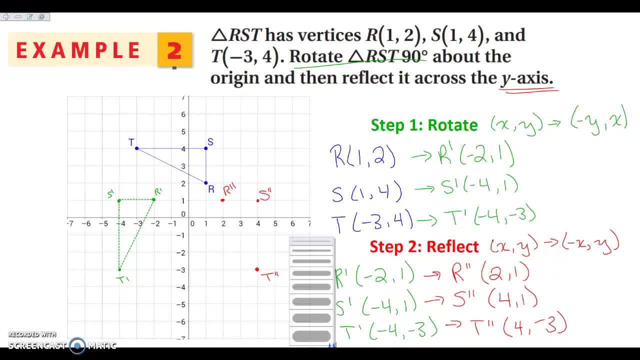 So this is my final image. So I'm going to make sure it is not dotted And I'm going to draw it just a little thicker. This one I'm not going to shade in, but you could if you wanted to. So you're more than welcome to shade or not. 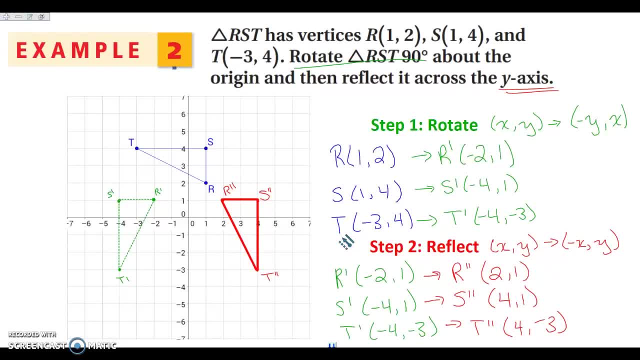 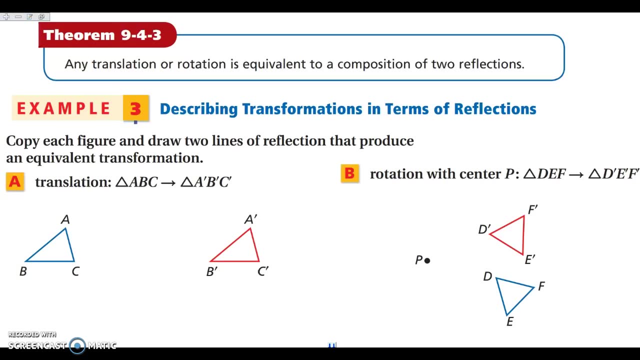 Just make sure it's clear which one is your final image. All right, If you have any questions about that, go ahead and write it down now. Okay, What we're looking at here is a translation, or a rotation can be found by doing two reflections. 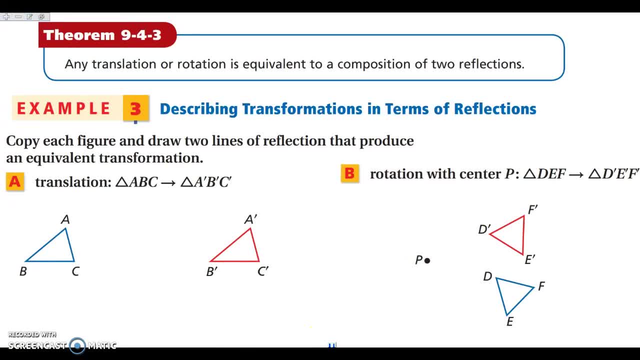 Okay. So what I'm looking at here is: I want to find where the lines of reflection would be. So what happens is, if I look at A to A prime, Okay, And now you have these steps listed out on the side of your notes. 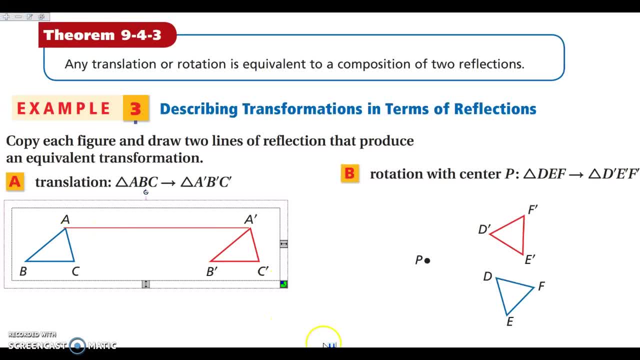 Okay, I'm going to look at A to A prime And I'm actually going to go ahead and make this. Come on, I just want this one, Whoopsies, Try and grabbing the right thing here, Just that, Thank you. 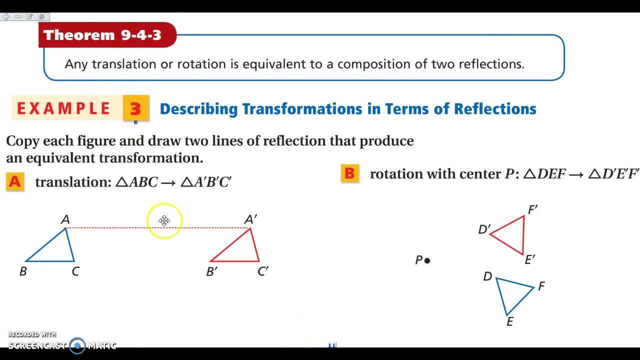 I'm going to go ahead and make this dotted. Okay, So I'm going to find this segment A to A prime- And what I'm going to do is I'm going to go ahead and try and estimate here where the center is. So this would be the midpoint for A to A prime. 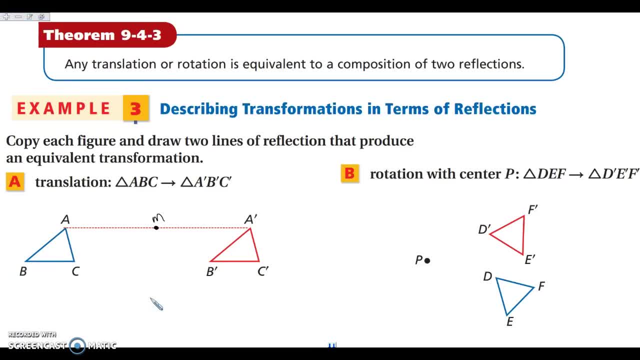 Okay, Again, I'm not actually measuring, I am just guessing to see about where it's going to be. This is all I'm really looking for you to do as well. I'm not looking for you to have exact measurements, Okay. 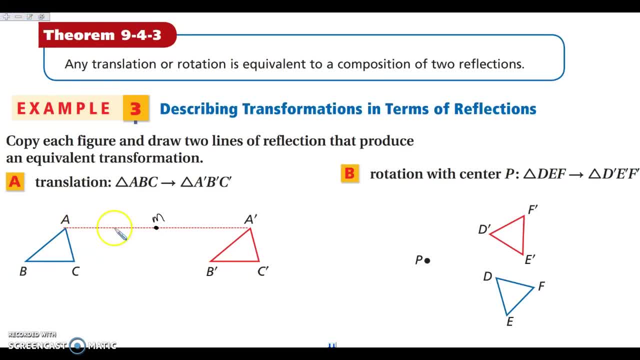 So then I'm going to look for the midpoint here, which is about here, And the midpoint over on this side, which is about here. So what I'm going to do from there is draw those two lines Here. Oops, A little crooked. 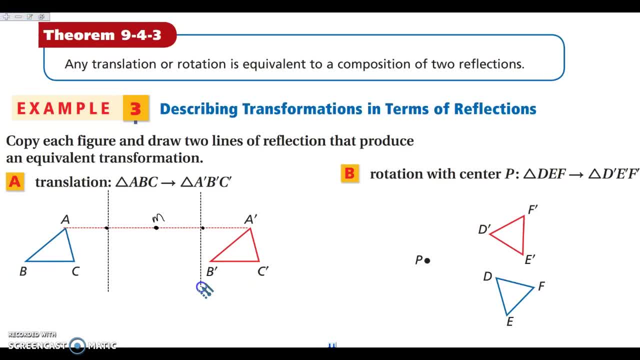 And here And miss the dot. So let me get those kind of fixed a little bit here. Shimmy that over And shimmy that over. Okay, So what happens is if I take this triangle here, ABC, and I reflect it over this line, 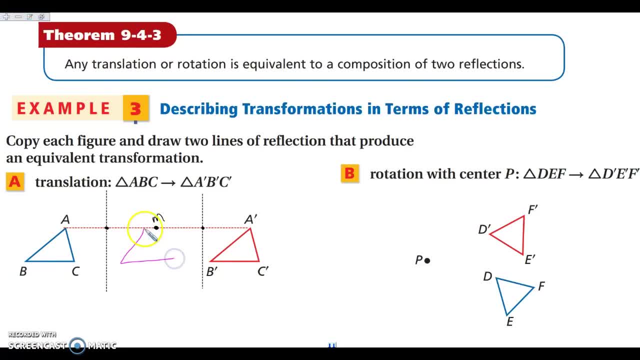 it's going to look about like this: Okay, Again, I'm sketching, I'm not even really looking, I'm just working really hard at it. Okay, But it'll look about like this. Then let's see if I can get that a little better. 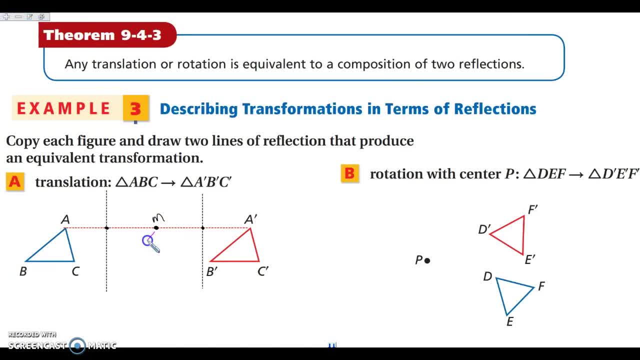 Okay, Here It's actually going to. it should be about here and here and here and here. Okay, So this is about where my reflection for ABC is going to be. Then, if I reflect that again over this line, I end up at A prime. 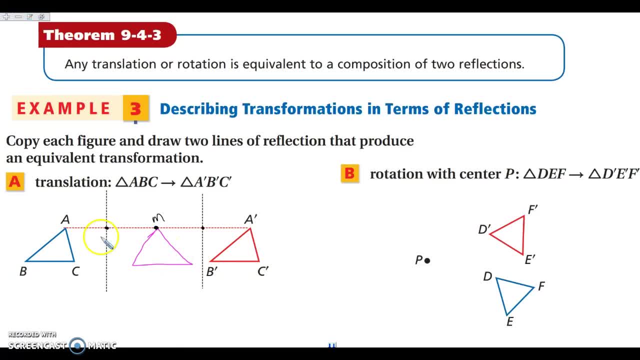 B prime, C prime. So that's what this is talking about. If I reflect, if I reflect this twice over parallel lines, then I'm ending up. beginning to end is just a translation. So when I reflect over two parallel lines, I have a translation. 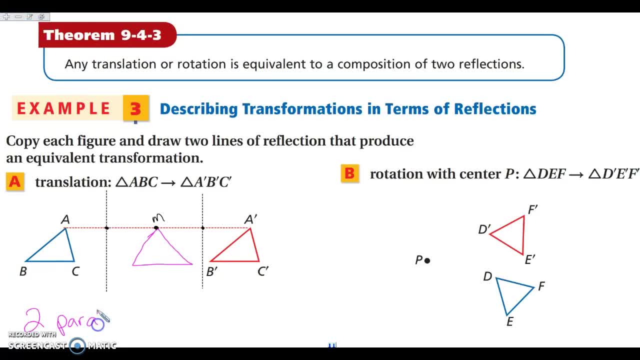 So two parallel lines, lines gives you a translation Okay. Okay, Then we're going to look over here, we're going to reflect again over two parallel line or, excuse me, over two lines, but this time we're going to intersect those lines. 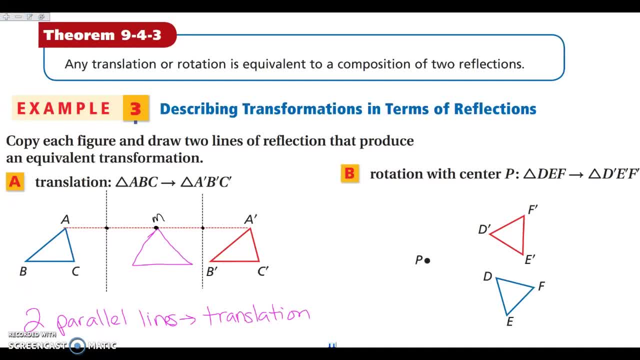 So the first thing that I'm going to do is I'm going to draw angle D, prime P, D, All right, And just like I did over here, I want to find the middle. So I'm doing that angle by sector right. 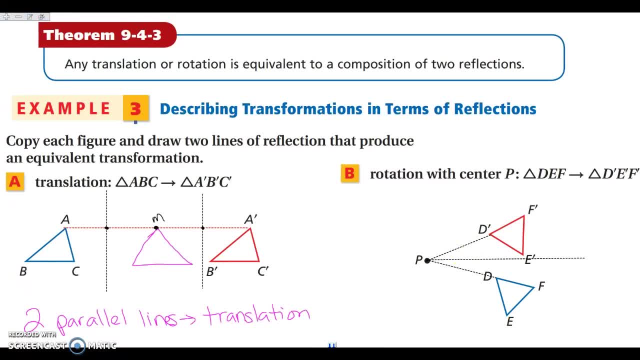 Again, I'm pretty much guesstimating Here. I'm looking to see: are these close? and then I'm going to bisect. each one of these totally missed the point on that one. Let me grab one more here. Try that again. 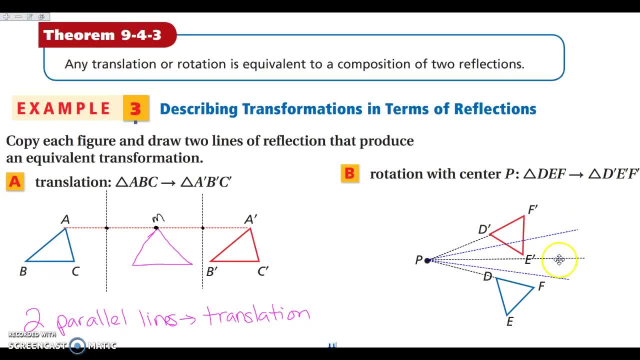 So if I were to kind of ignore these lines, this one and this one and this one, now don't erase them from your paper, but I just kind of wanted to show you I can't grab that one. Come on, Let me do that. 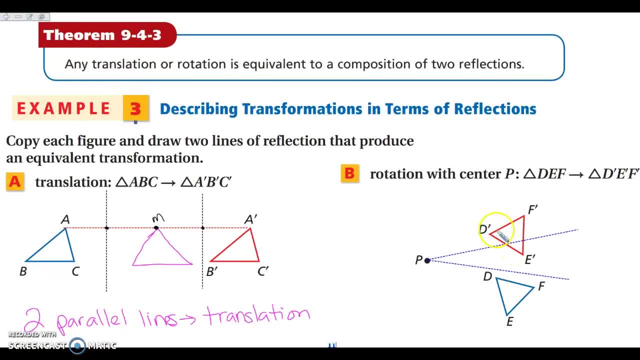 So I'm going to go ahead and draw a triangle and then I'm going to duplicated What it's going to look like here. If I reflect this triangle, let's do D, E, F over this line. I'm going to be looking somewhere right in here. 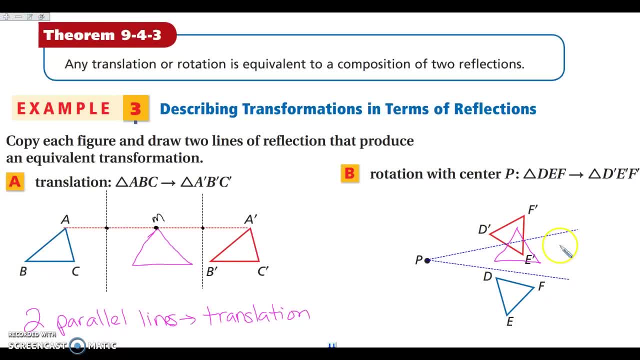 Okay, Not exactly, but kind of close. Then if I reflected again over this line, it's going to flip up and land on top of this one. So two reflections. when your lines intersect, I'm going to do a triangle over this one. 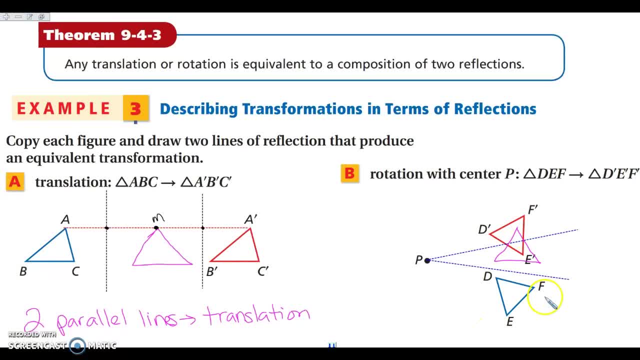 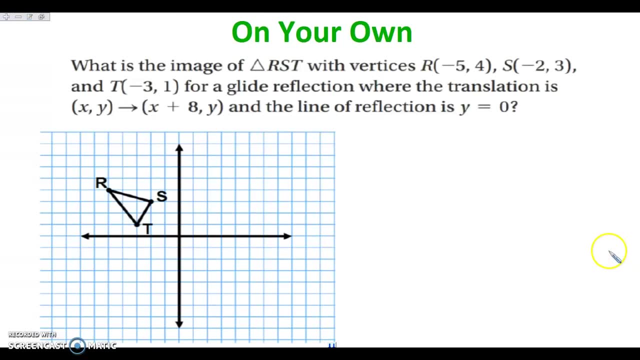 intersect are going to give you a rotation, so I'm rotating this this way, all right. so that's what you need to remember is: two intersecting lines are a rotation, two parallel lines are a translation. so what I would like for you to go ahead and do is pause the video and try this one. 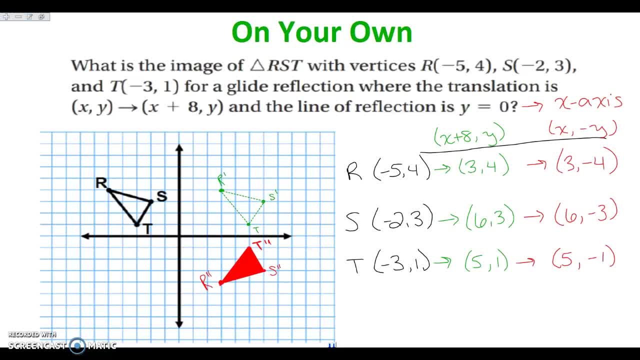 on your own. okay, so you may need to pause the video to kind of check your answers here. notice that I wrote down points r, s and t. then in green I wrote my first transformation, which was a translation, and then in red I wrote my second translation, or transformation was a reflection. 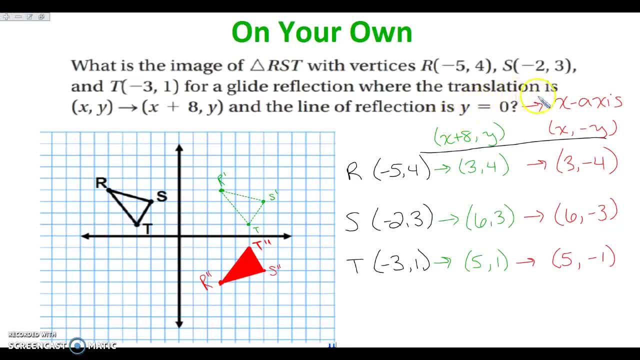 over the line y equals zero. please realize that the line y equals zero is the x-axis, because every y value on this line is zero. okay, so please write down any questions you have about that and I will see you guys in the next video In class. have a wonderful day.